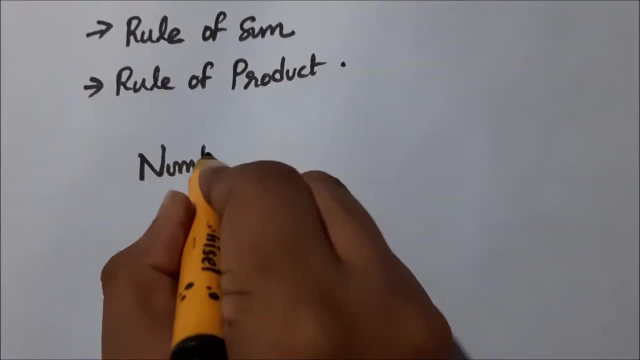 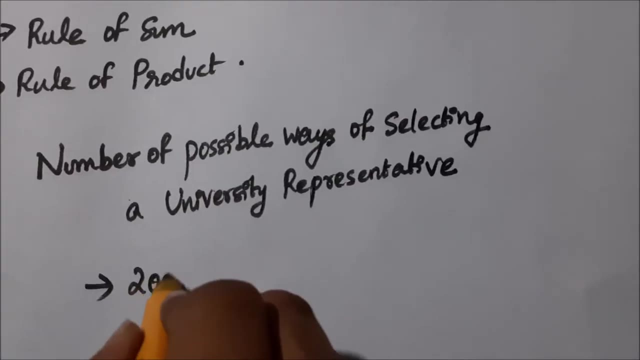 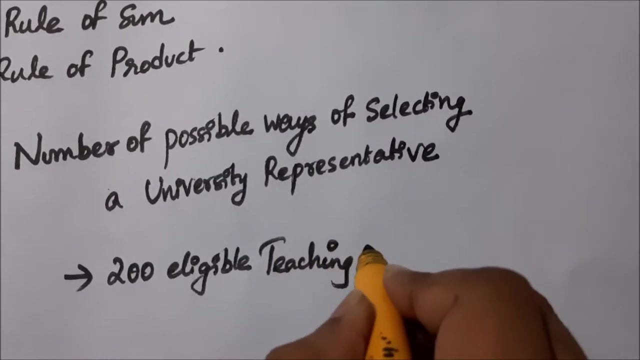 So let's understand the rule of sum using an example. Okay, so here we are interested in finding the number of possible ways of selecting a university representative. Now, a university representative can be either a teaching staff or a non teaching staff. There are 200 eligible teaching staff. 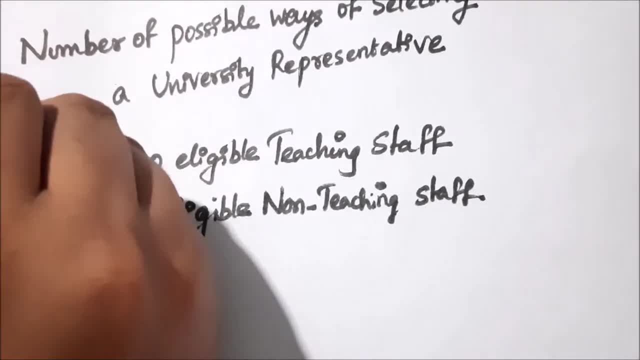 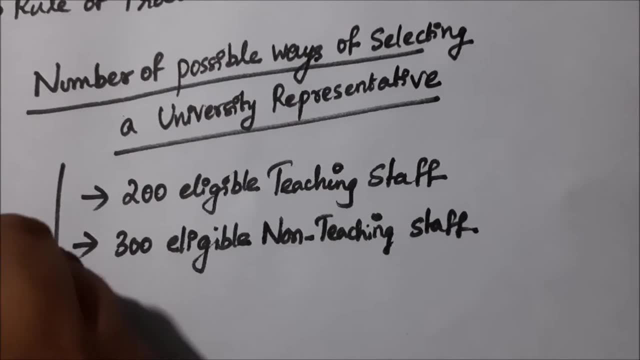 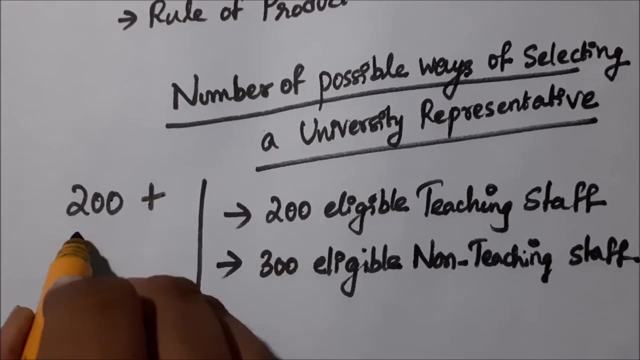 and three 300 eligible non-teaching staff. So any one among the 200 eligible teaching staff can be a university representative, or any one among the 300 eligible non-teaching staff can be a university representative. So when we are interested in finding the total possible ways of 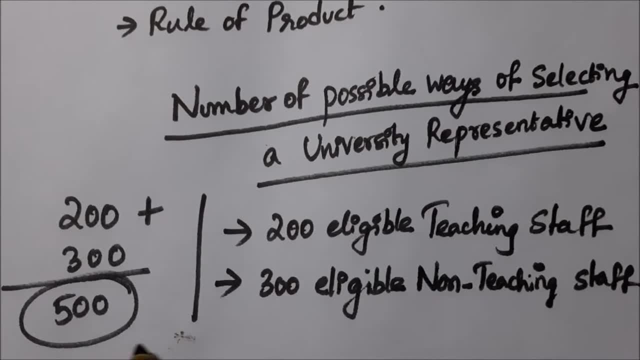 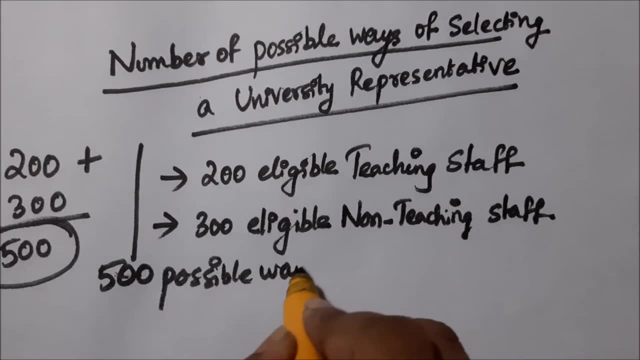 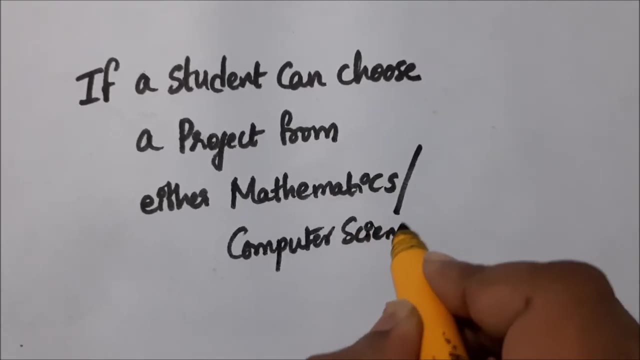 selecting a university representative, which is nothing but 200 plus 300, that is 500. So there are 500 possible ways to select a university representative. Okay, let's see another example. Suppose a student can choose a project from either mathematics or computer science. 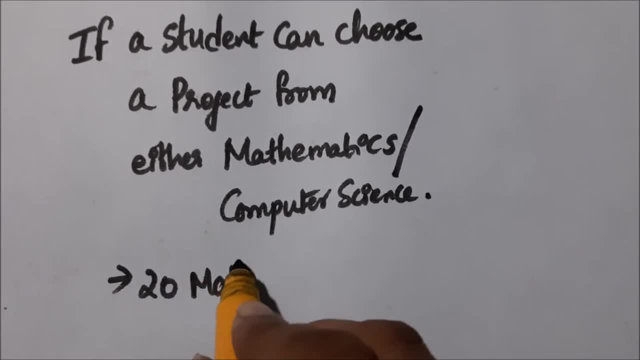 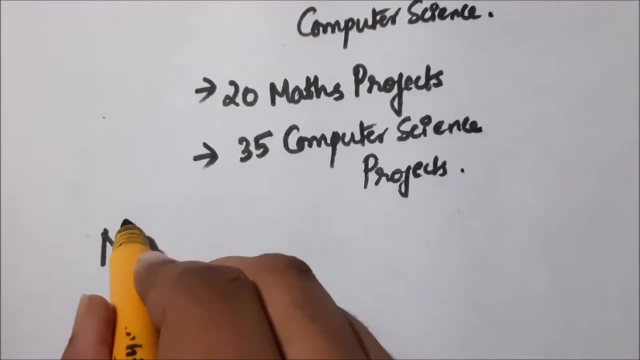 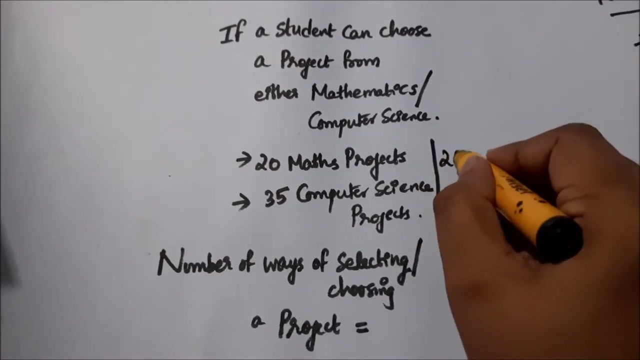 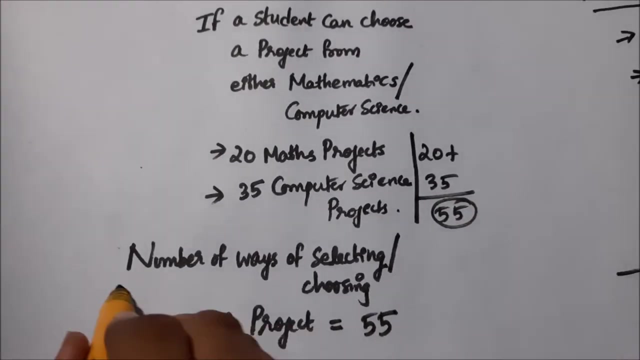 Now, given that there are 20 maths projects available and 35 computer science projects available, Now the number of ways of selecting or choosing a project is going to be 20 plus 35, which is 55. As any one among the 20 mathematics projects he can choose, or he can choose any one among the 35 computer science projects. 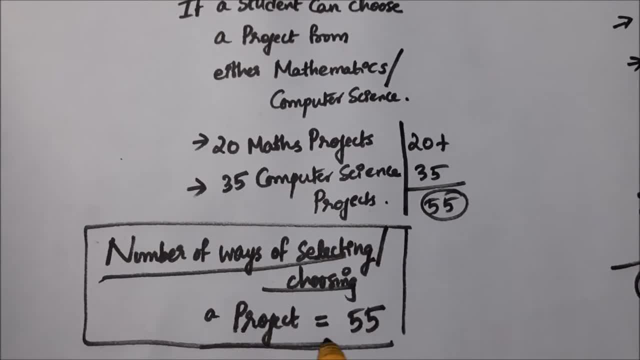 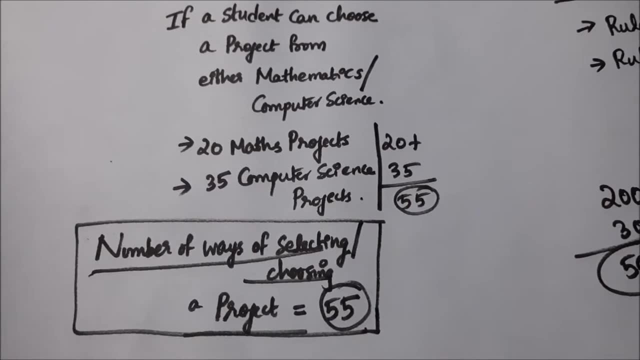 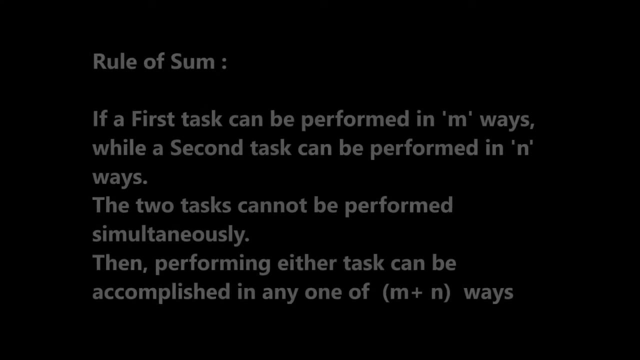 So when we count the total possible ways of choosing a project, that is going to be 20 plus 35,, which is 55.. Alright, now let's get into the formal rule of sum. Let's see what it says If a first task can be performed in m ways. 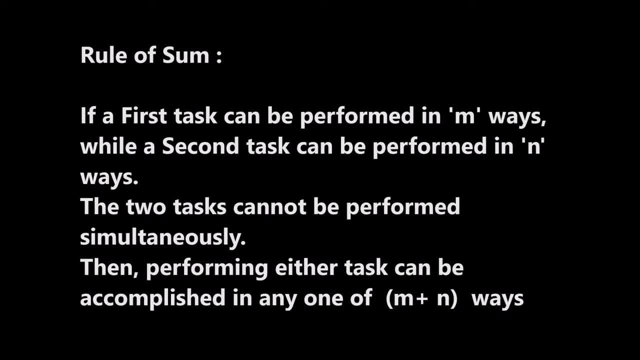 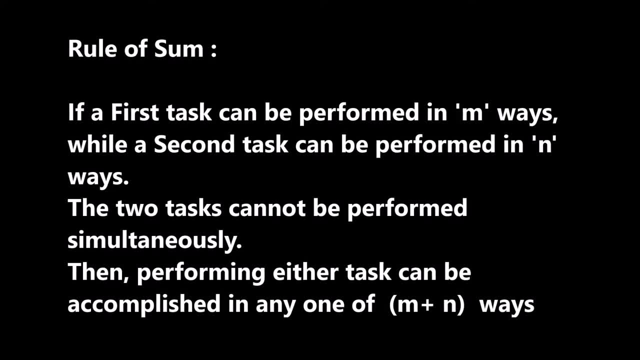 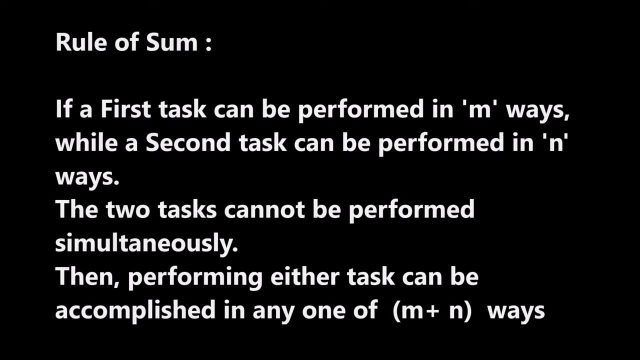 while a second task can be performed in n ways. Given that these two tasks cannot be performed simultaneously, That it means that the two tasks are not happening at the same time. Now, then, Performing either task can be accomplished in m plus n ways. Okay, So this is the rule of sum. 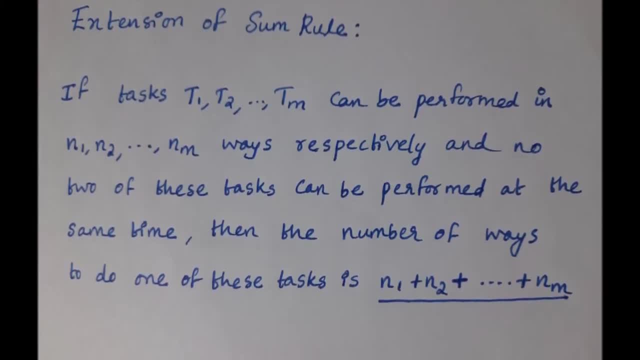 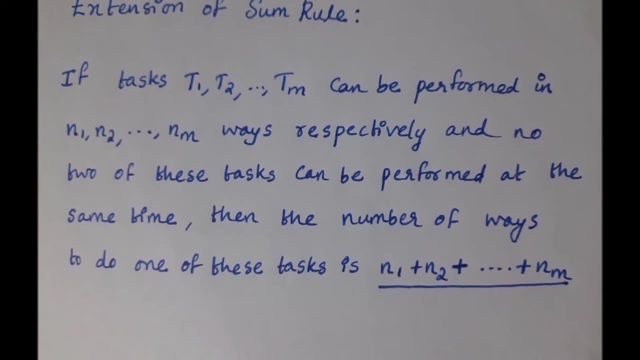 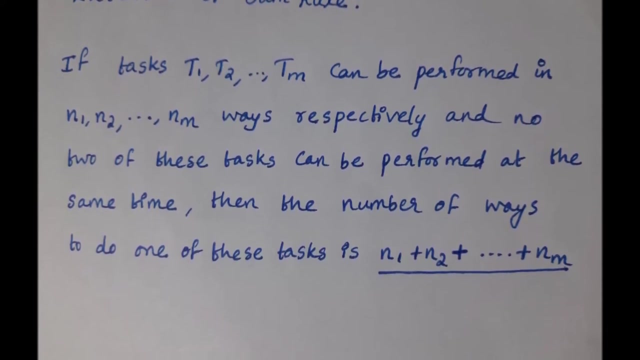 Now it is possible that the sum rule can be extended for more than two tasks, So if task t1, t2 up to tm can be done in n1, n2 and so on, up to nm ways respectively and No two of these tasks can be performed at the same time, 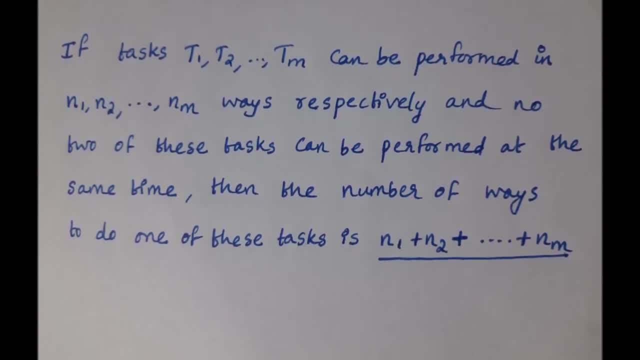 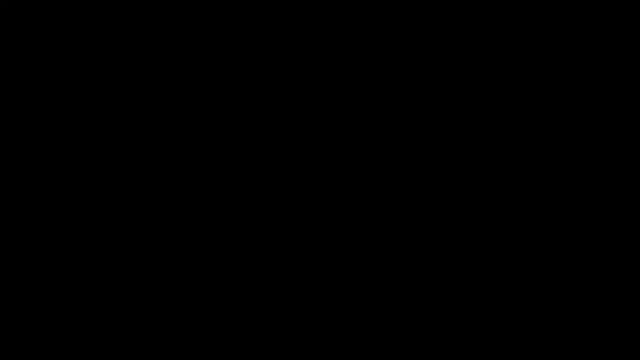 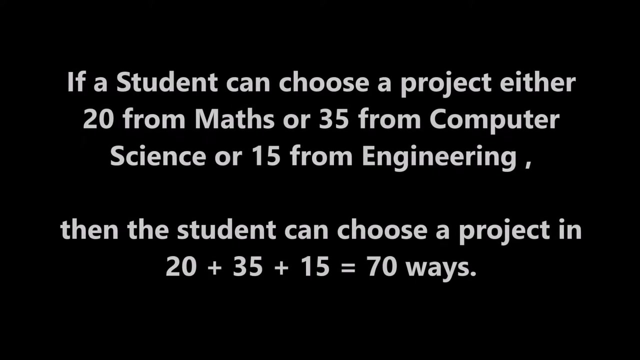 Then the number of ways to do one of these tasks is n1 plus, n2 plus and up to plus nm. So as an example, suppose if a student can choose a project, either 20 from mathematics or 35 from computer science, or 15 from engineering. 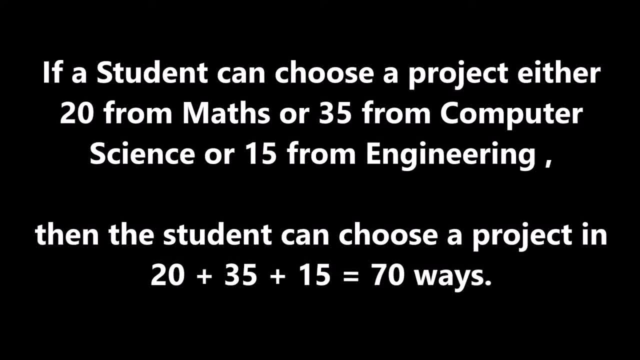 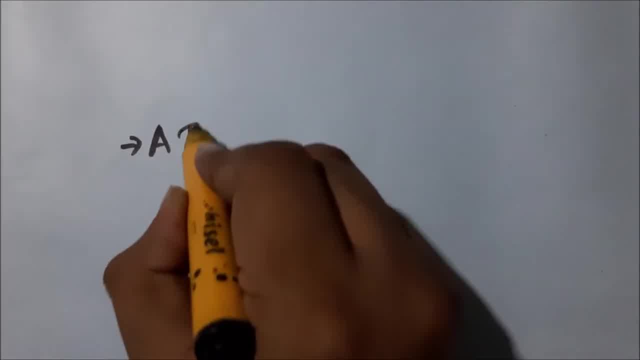 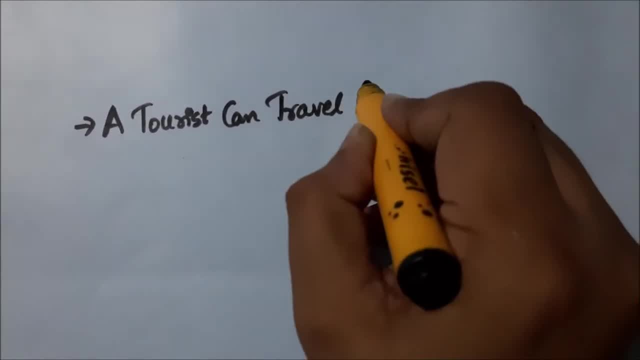 Then the student can choose a project in 20 plus 35 plus 15, which is 70 ways Alright. so now let's get into some examples where we apply the rule of product. Okay, suppose a tourist can travel from Palakkad to Karnataka. 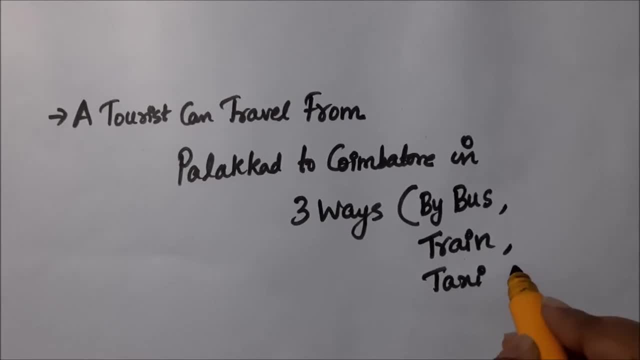 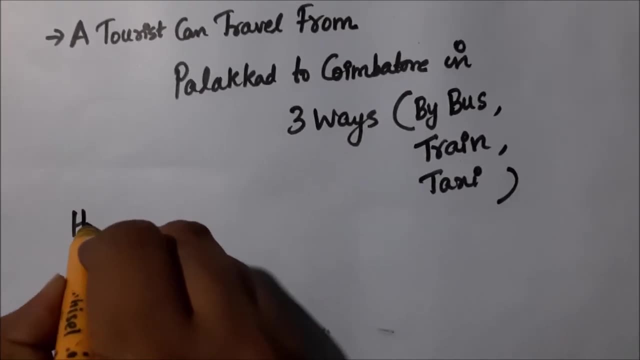 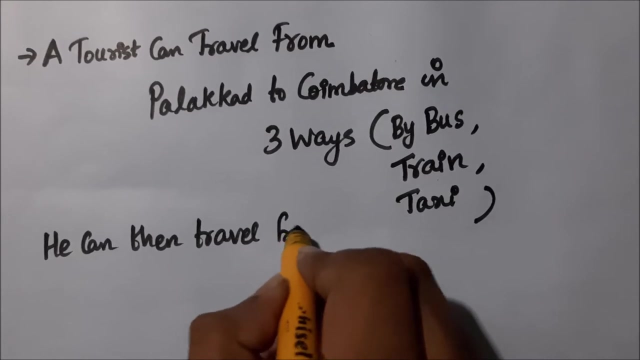 to Coimbatore in three ways: By bus, or by train or by taxi. So these are the three ways a tourist can travel from Palakkad to Coimbatore. Okay, Now, so he has some business in Coimbatore to do now. after that he has to go to Chennai. 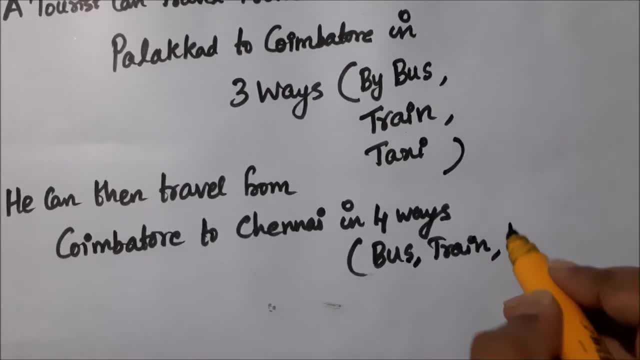 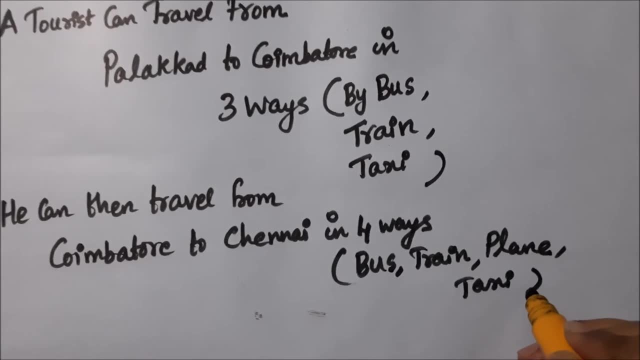 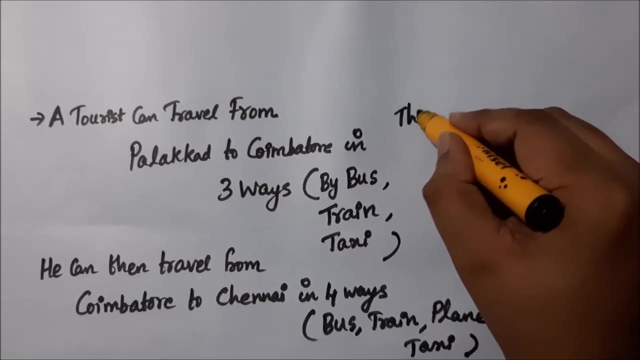 So he can then travel from Coimbatore to Chennai in four ways. He can either take bus or by train, or by aeroplane or by taxi. so, again, from Coimbatore to Chennai, He has four ways of going. Okay, So the question is, the tourists can travel from Palakkad to Chennai in how many number of ways? 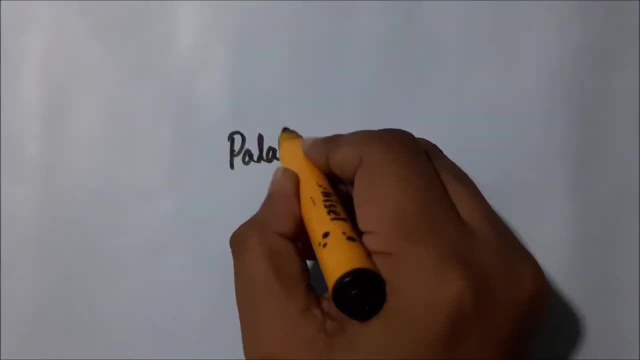 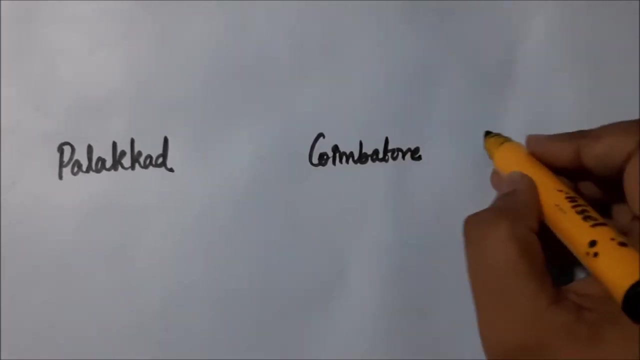 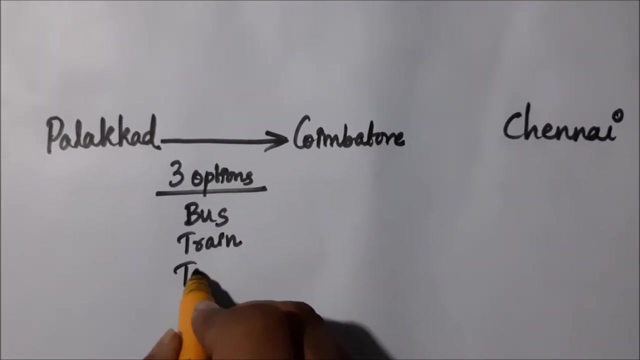 Okay, that is the question. Let's see. his journey starts at Palakkad and Intermediate stop is Coimbatore and the final destination is Chennai. Alright, now there are three options of going from Palakkad to Coimbatore: bus, train and taxi. These are the three options. 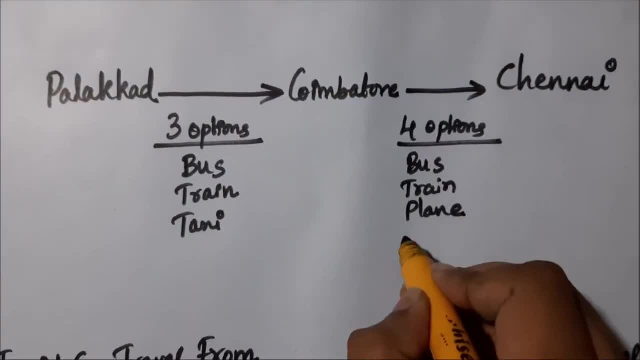 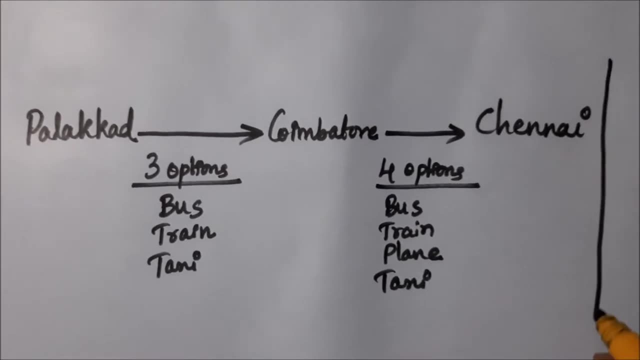 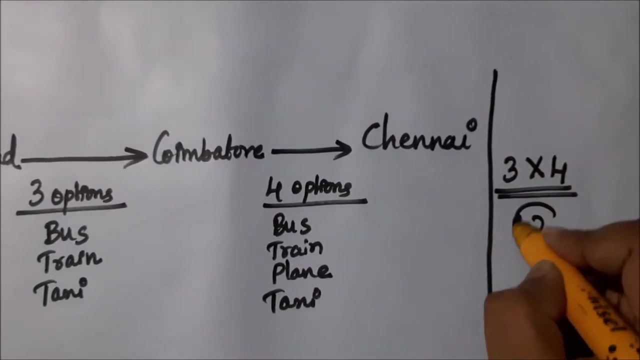 from Coimbatore to Chennai, and there are four options: bus-train, plane and taxi. So we want to calculate the number of possible ways of traveling from Palakkad to Chennai for that tourist. Alright, Now the answer is going to be three into four: 12. 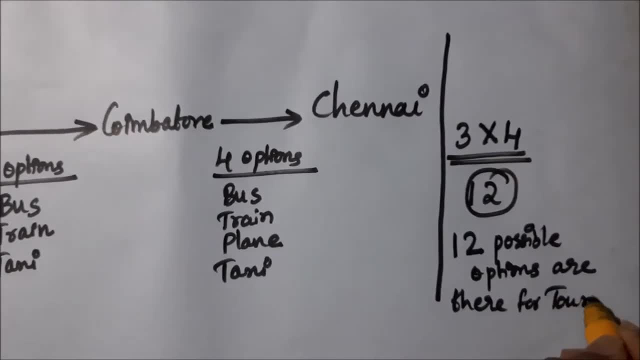 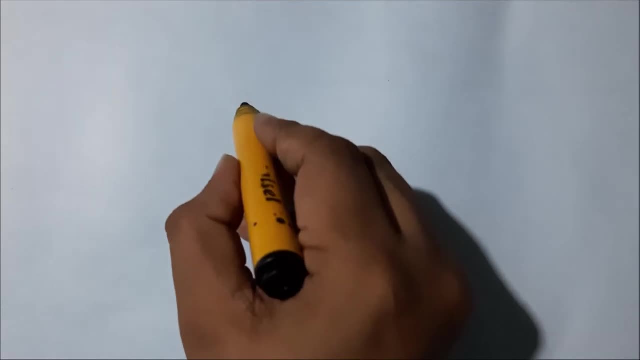 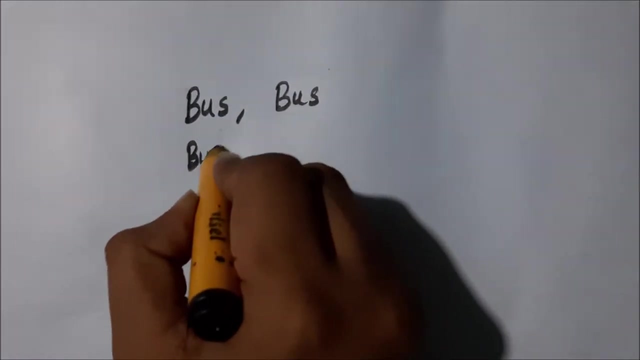 that are 12 possible options for the tourist. Now, when we enumerate or list out the total possible options, It is going to be like this: In the first journey he'll take the bus and in the second journey he's going to take the bus, Bus, train bus, plane bus. 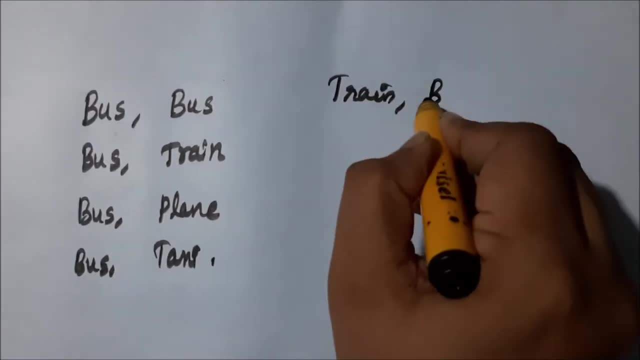 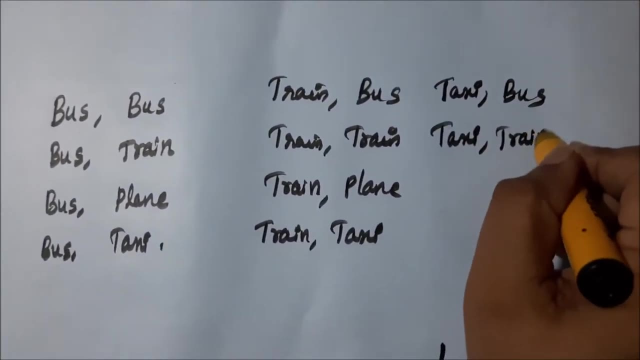 taxi train, bus, train, train, train plane, train, taxi, taxi bus, taxi, train, taxi, plane, taxi taxi. So you can see that for each of the available options of traveling from Palakkad to Coimbatore, 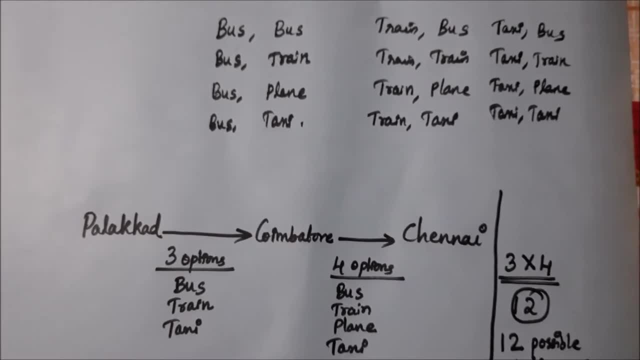 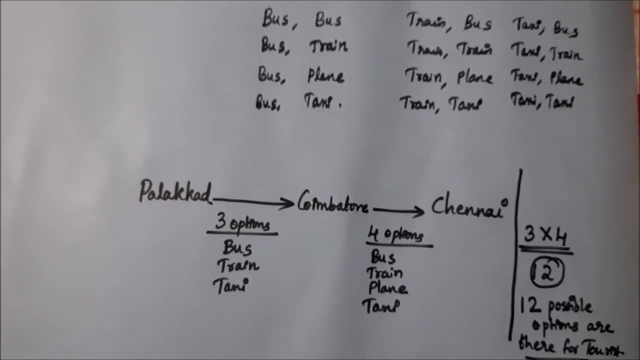 the tourist has four options available for traveling from Coimbatore to Chennai. This is the case for the each of the option of traveling from Palakkad to Coimbatore, and there are three options. So that is why the total number of possible ways is going to be 3 into 4, which is 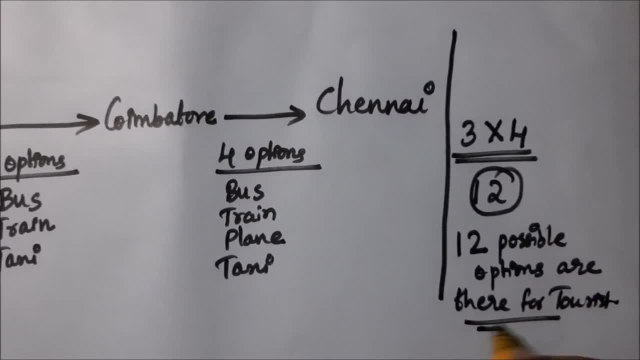 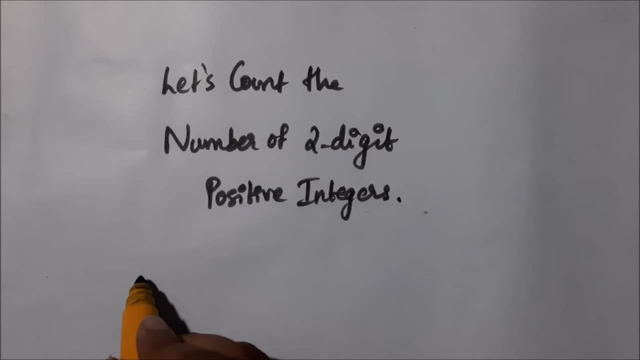 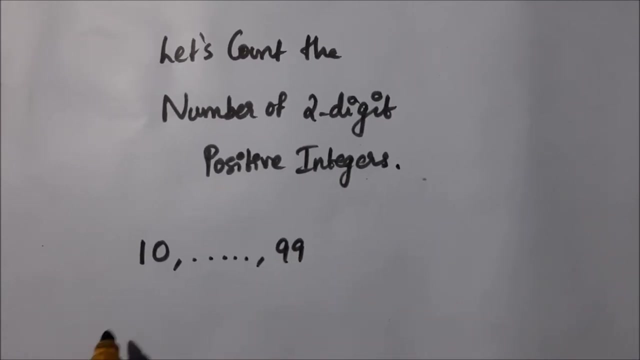 12, and this is exactly an example of a product rule. Let's see one more example. So let's count the number of two-digit positive integers. That is very simple, right? We know that the two-digit first two-digit positive integer is going to be 10 and the last two-digit positive. 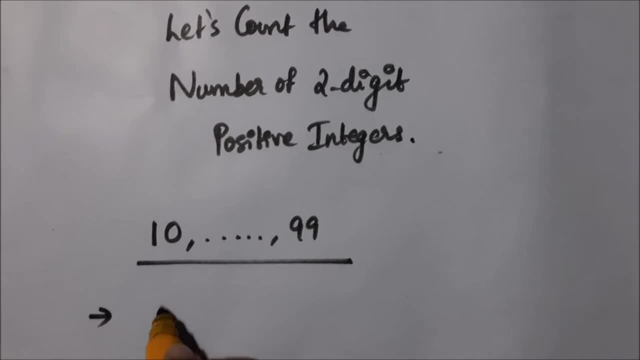 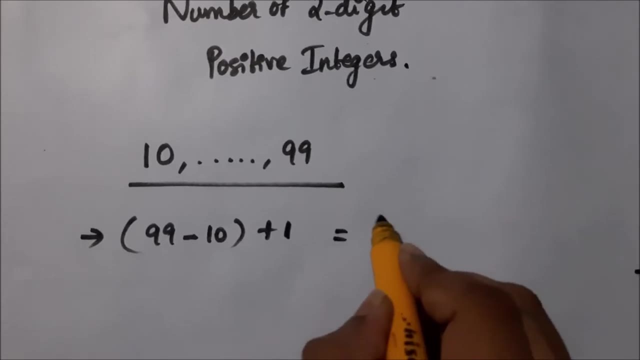 integer is going to be 99.. So, from 10 to 99, including both 10 and 99, there are 99 minus 10 plus 1, 90 numbers. So the number of two-digit positive integers is going to be 90.. As we can, 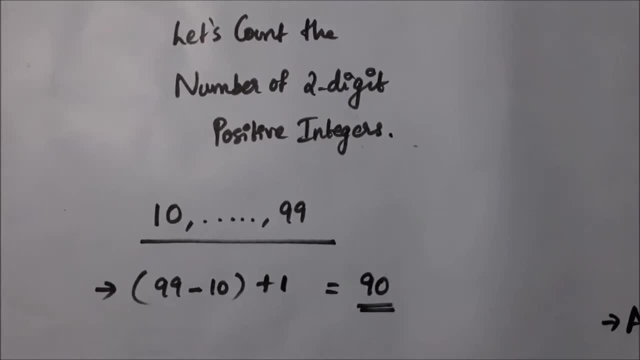 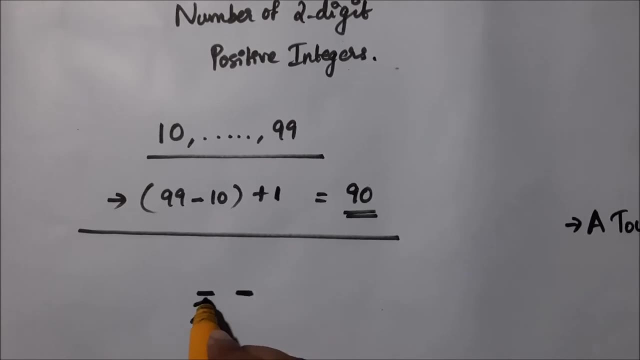 see if we count this way. it is a very easy method of counting. Now let's see another way of counting where we can apply our product rule. So we are focused on counting the number of two-digit positive integers. So there are two-digits. 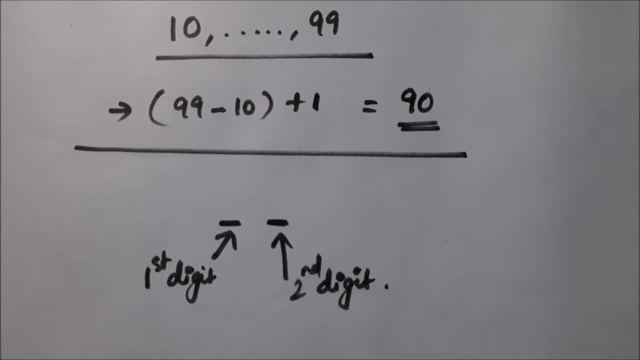 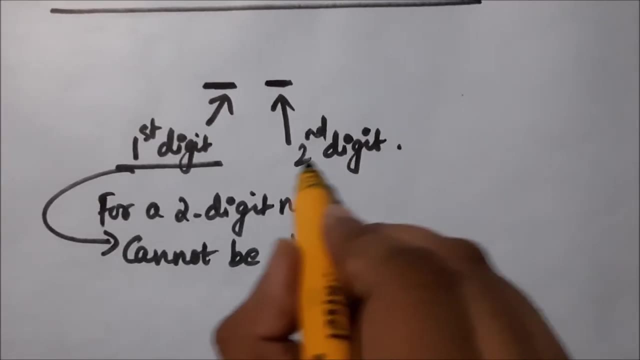 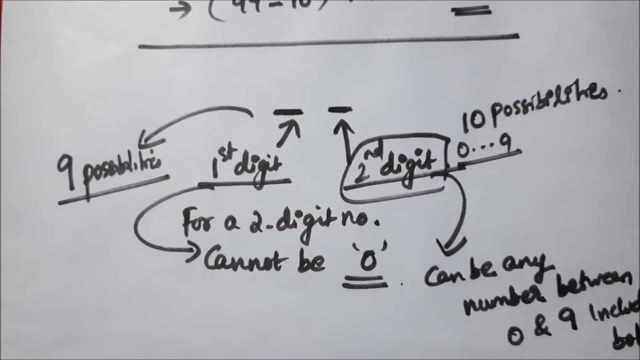 first digit and second digit. Let's mark it this way: Now we know that when we are considering two-digit numbers, the first digit here cannot be 0, right, That's the leading number. or the 10th place number, That cannot be 0.. Now for the first digit. there are 9 possibilities. 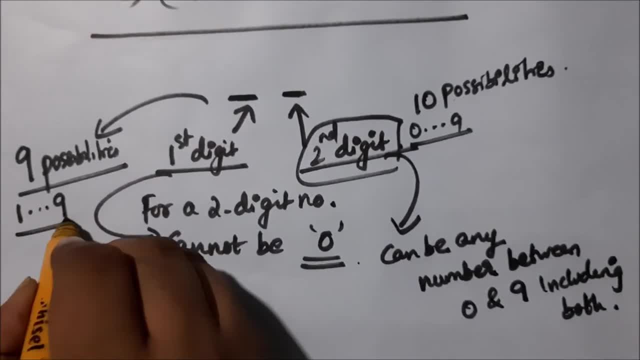 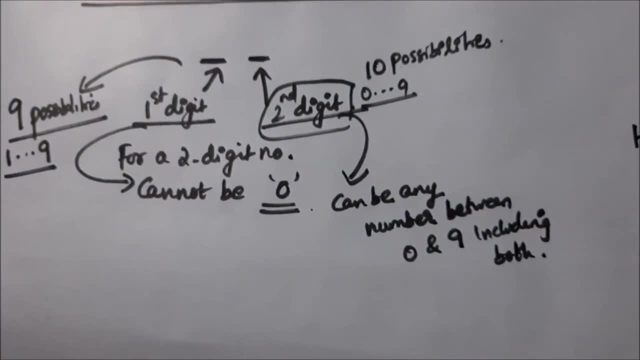 It can be any number from 1 to 9.. So there are 9 possibilities For the first digit. Second digit can be any number between 0 and 9, including 0 and 9.. So there are 10 possibilities for the second digit. Now we know that there are 9 possibilities. 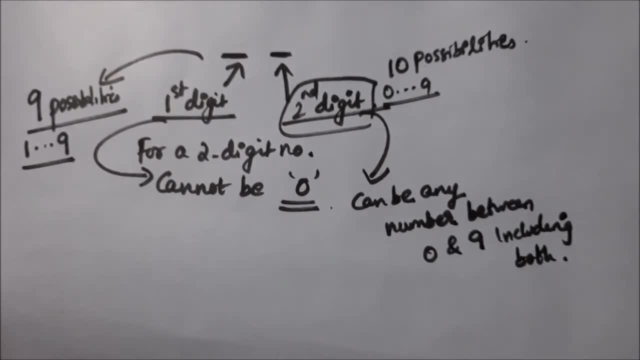 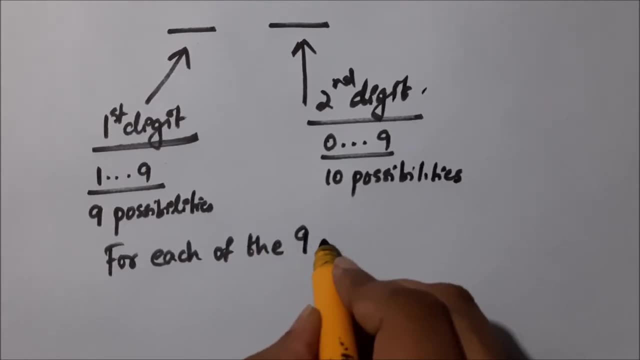 for the first digit and there are 10 possibilities for the second digit. Now we say that there are 9 into 10, 90 possibilities for such two-digit numbers. It is because for each of the 9 possibilities for the first digit, 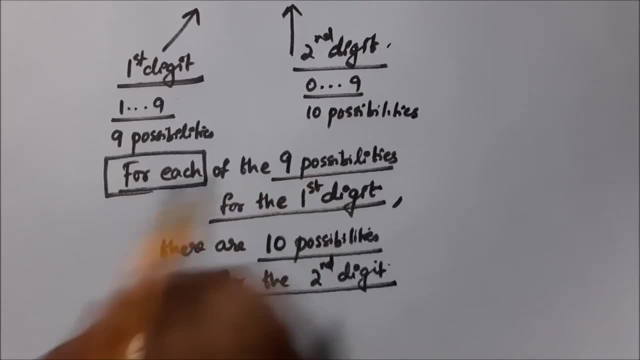 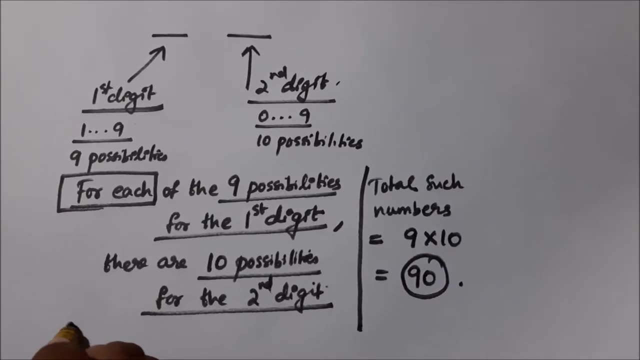 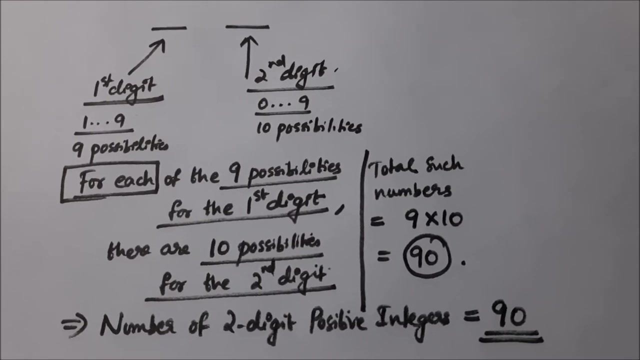 There are 10 possibilities for the first digit. There are 10 possibilities for the second digit. That's why we have number of two-digit positive integers equal to 9 into 10, which is 90. And that's how we applied the product rule here. So now let's say what the rule of product 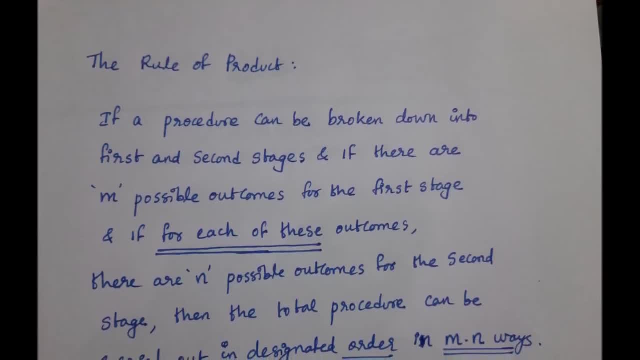 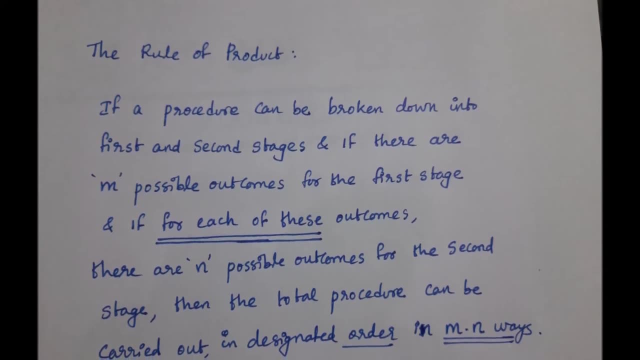 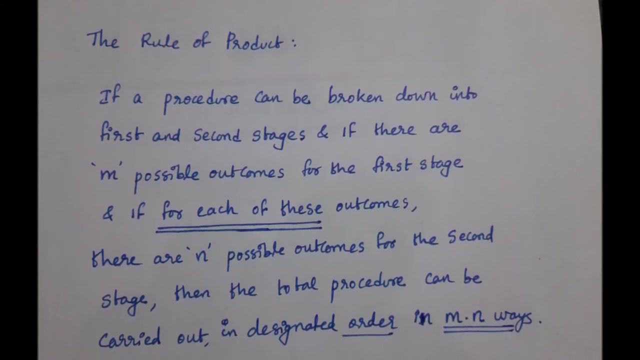 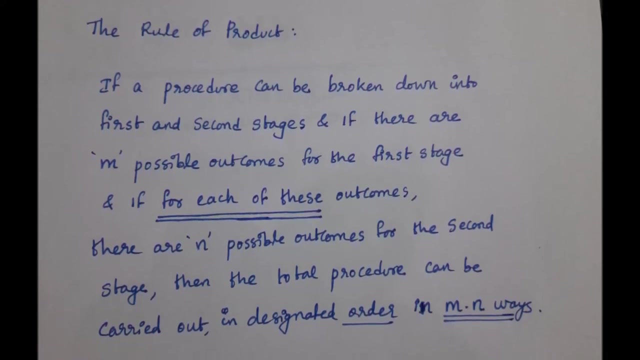 formally says. The rule of product says that if a procedure can be broken down into first and second stages and if there are M possible outcomes for the first stage And if, for each of these outcomes, there are N possible outcomes for the second stage, Then the total procedure can be carried out in the designated order MN ways. 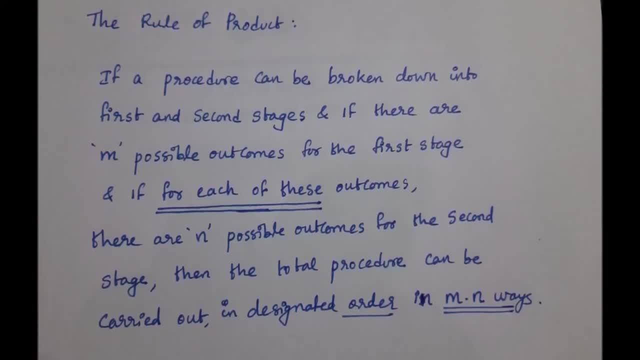 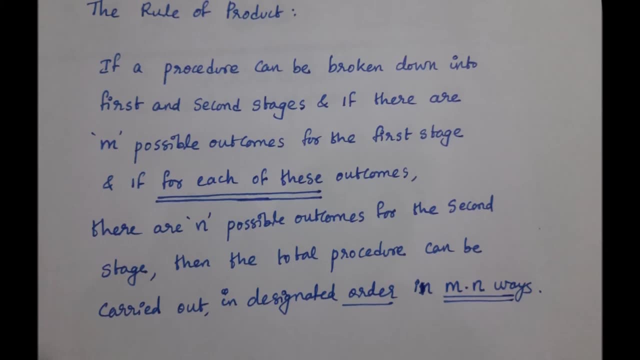 The important part is that If for each of these outcomes there are n possible outcomes, then there are MN ways. So for each of the M possible outcomes in the first stage, there are n possible outcomes in the second stage. That's why the total number of ways is MN. 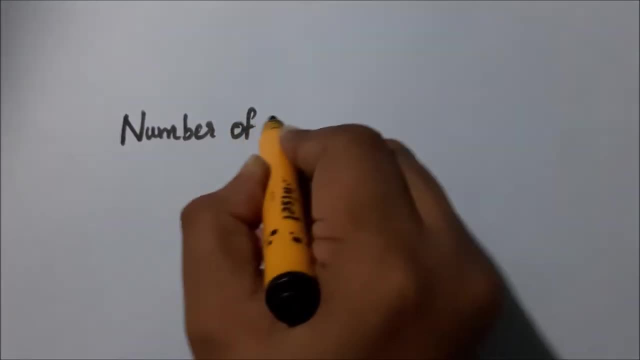 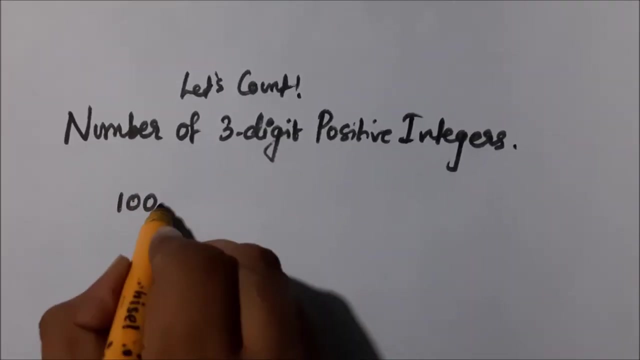 Now for the next one. Let's say that the total number of ways is MN, As there was an explanation, then the total for the sum rule. there is an extension for the product rule also. Let's see an example for that. Let's count the number of three-digit positive integers, So the 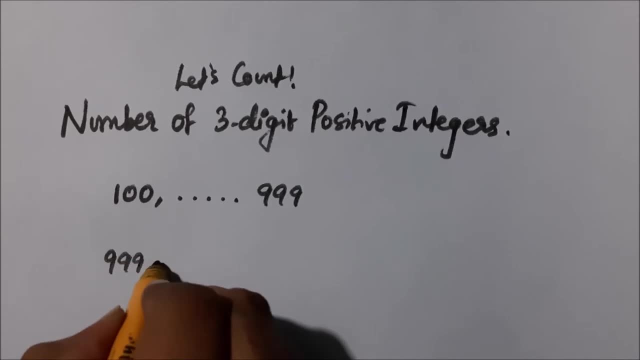 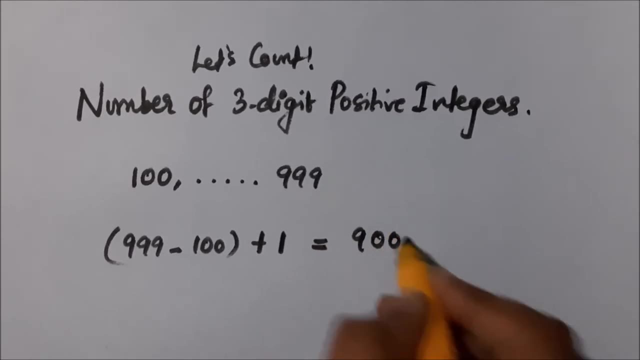 first three-digit positive integer is 100 and the last three-digit positive integer is 999.. Now we can easily count the number of three-digit positive integers this way: 999 minus 100 plus 1, which is 900.. Now we want to apply the 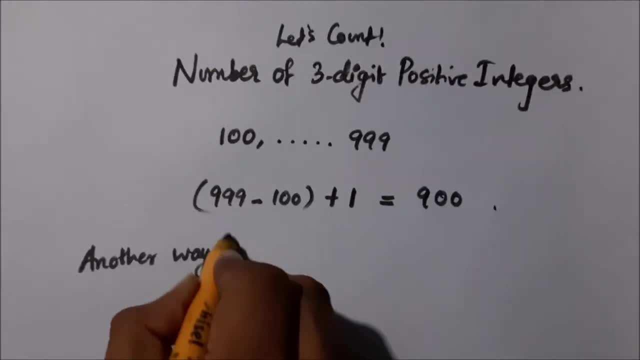 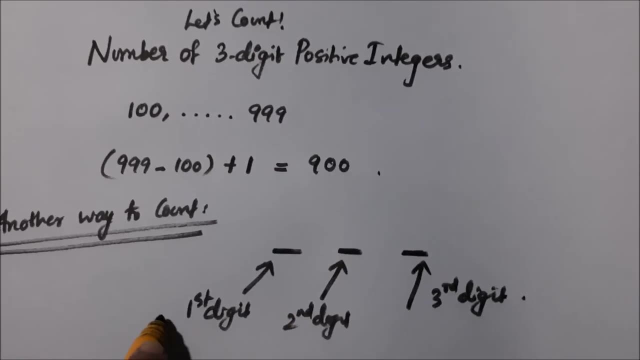 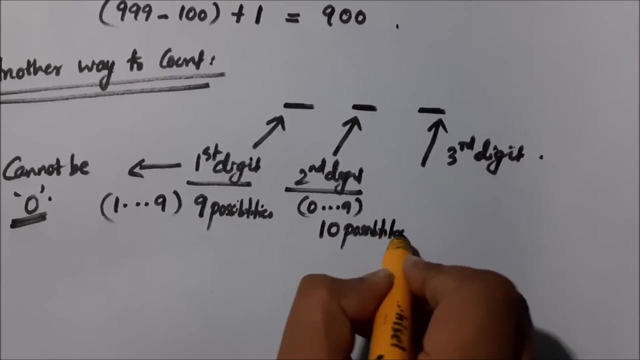 product rule. So let's see another way to count this. Now there are three digits right: first digit, second digit and third digit. let's mark it this way again: first digit cannot be 0. right Now there are nine possibilities for the first digit. any number from 1 to 9, including 1 and 9, can be a possibility for the first digit. 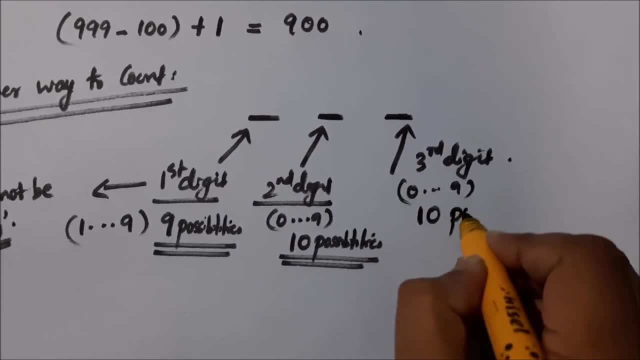 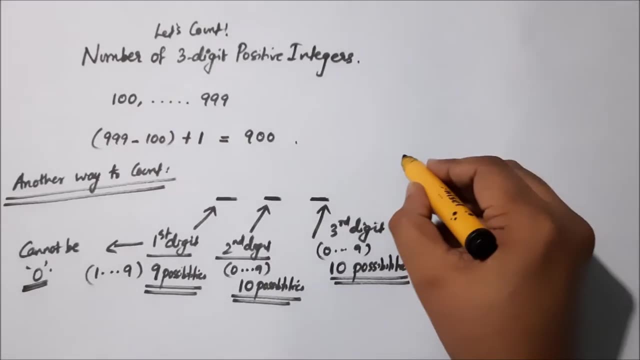 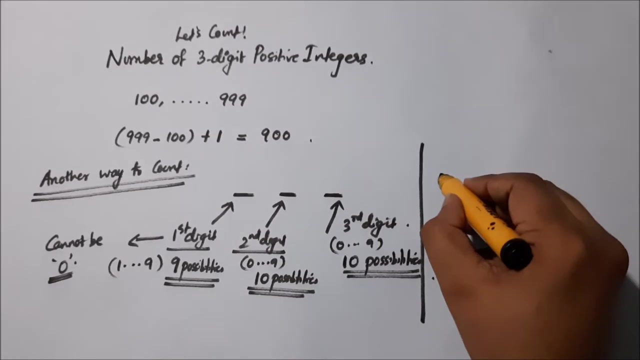 So first digit has nine possibilities. second digit have 10 possibilities and the third digit have 10 possibilities. Alright, now for each of the nine possibilities. for the first digit, there are 10 possibilities for the second digit, Meaning that there are 90 ways we 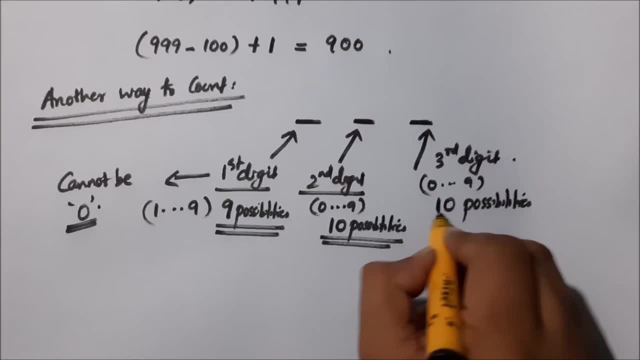 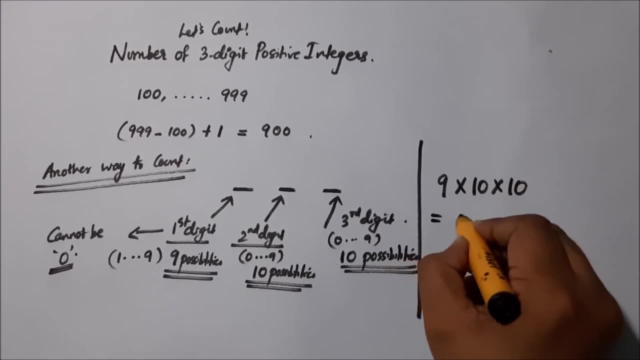 can arrange the first two numbers. Now, for each of these 90 first two digit numbers, there are 10 possibilities for the third digit right, Meaning that 90 into 10 900 numbers are there. That's how we apply the product rule. 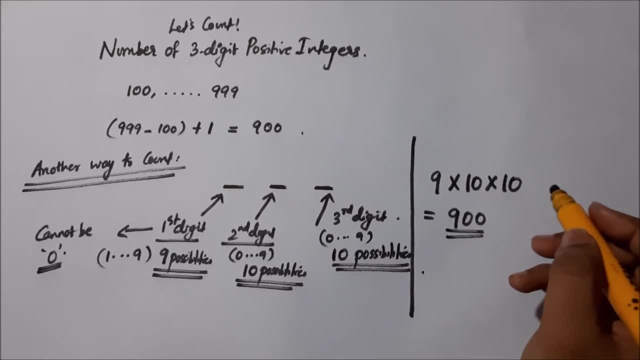 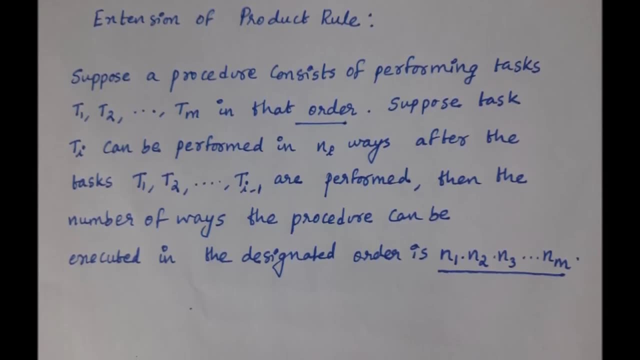 And this is an example for the extension of the product rule. Let's see what it says. Suppose a procedure consists of performing task T1, T2 and so on up to Tm in that order. Suppose task Ti can be performed in Ni ways. after the: 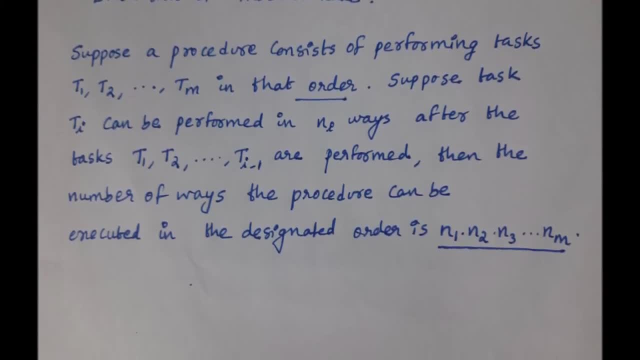 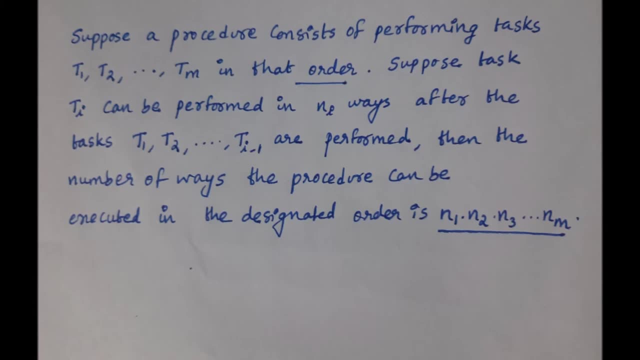 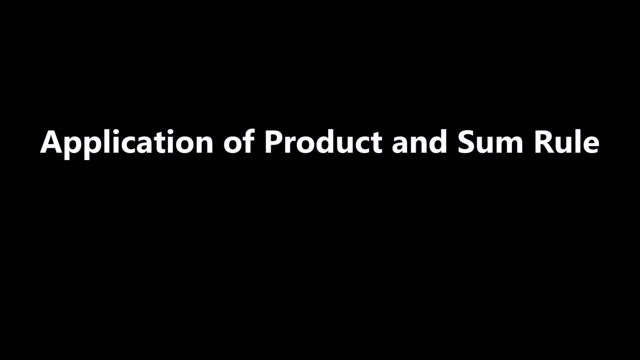 task T1, T2 up to Ti-1 are performed, Then the number of ways the procedure can be executed in the designated order is N1 into N2, into N3, up to Nm. So now we have seen both rule of sum and rule of product and its 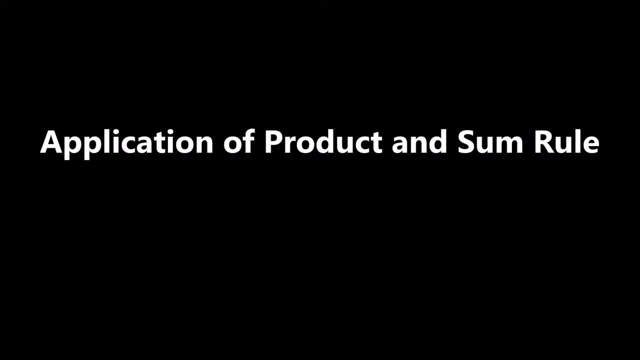 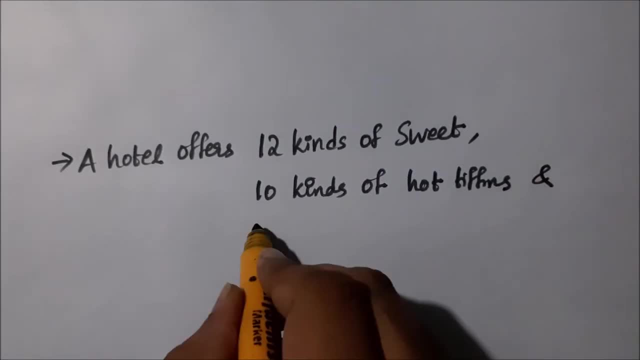 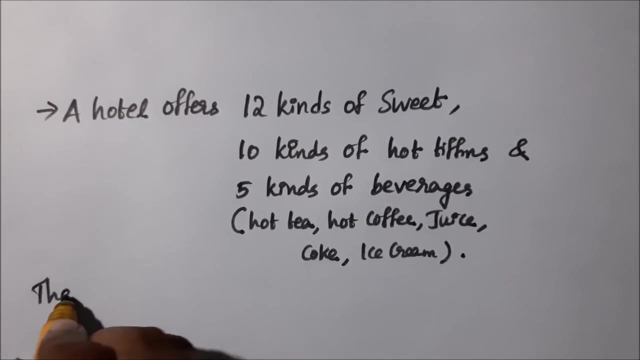 extensions and their examples. Now let's see an application of both product and sum rule. A hotel offers 12 kinds of sweet, 10 kinds of hot tiffins and 5 kinds of beverages. The five kinds of beverages are hot tea, hot coffee, juice, coke and ice. 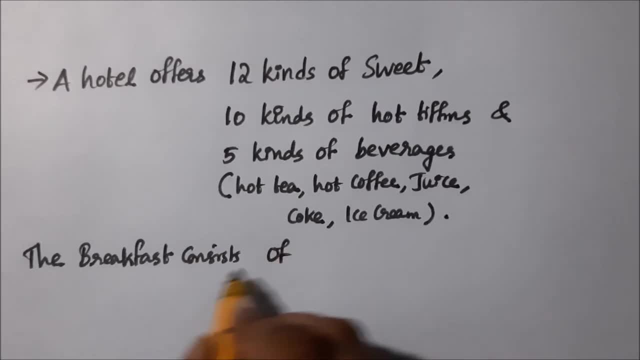 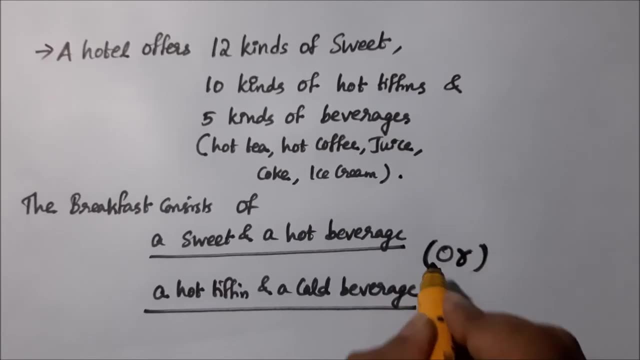 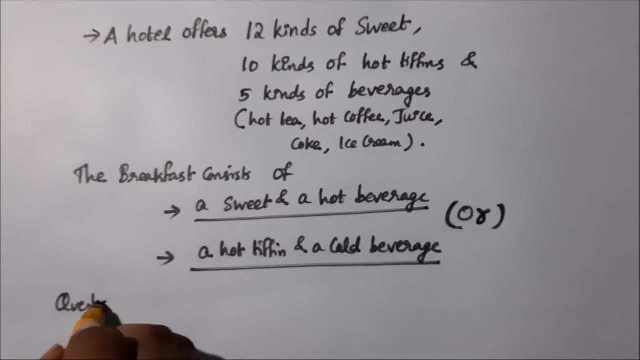 cream. Alright, the breakfast consists of a sweet and a hot beverage, or a hot tiffin and a cold beverage. These are the breakfast menu. It can be a sweet and a hot beverage, or a hot tiffin and a cold beverage. The question is the number. 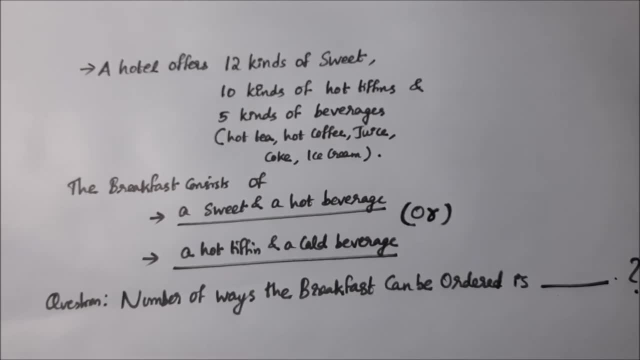 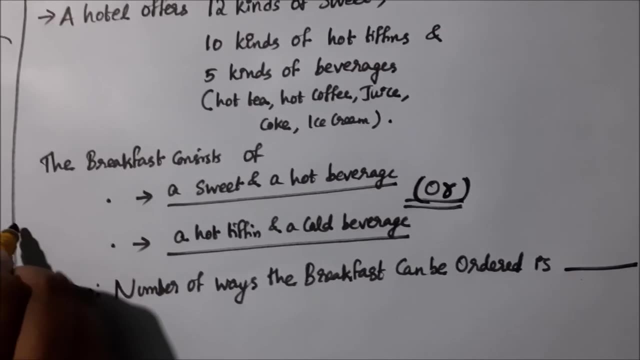 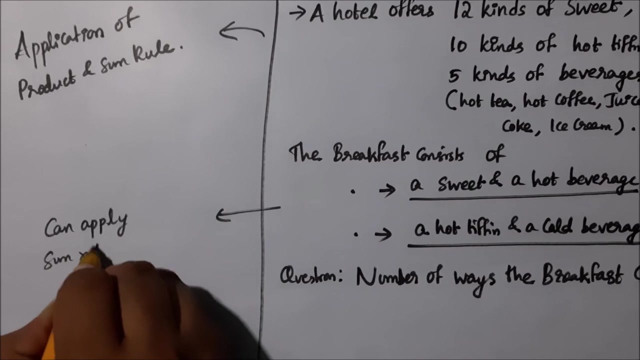 of ways the breakfast can be ordered is dash, So we want to find the number of possible ways we can order the breakfast. So breakfast is either a sweet, hot beverage or a hot tiffin and a cold beverage, Since there is, or we have the task 1 as a sweet and a hot beverage And task two as a hot. 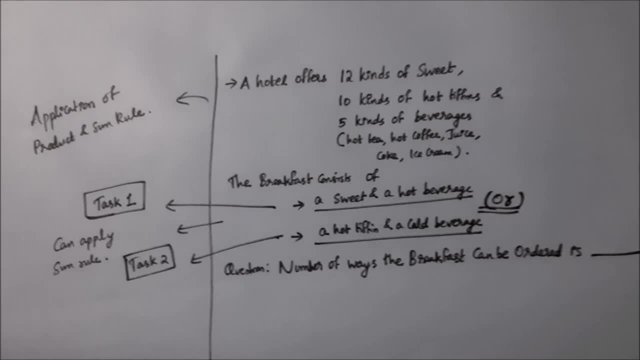 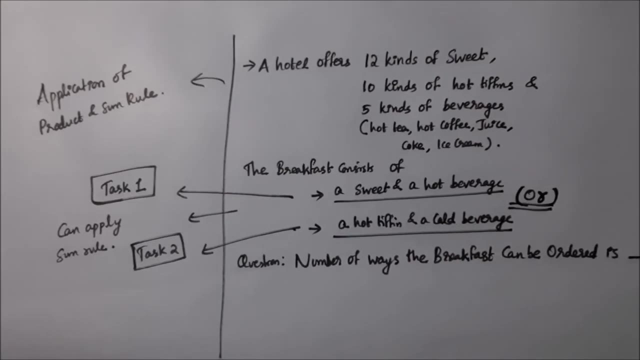 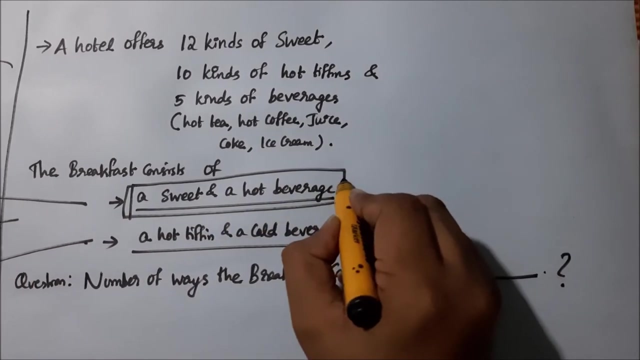 tiffin and a cold beverage. Now these task 1 and task 2, cannot happen simultaneously, Right, So we can apply the sum rule. Since there these are the two tasks that cannot be performed simultaneously, we can apply the sum rule. So now we want to find out how we